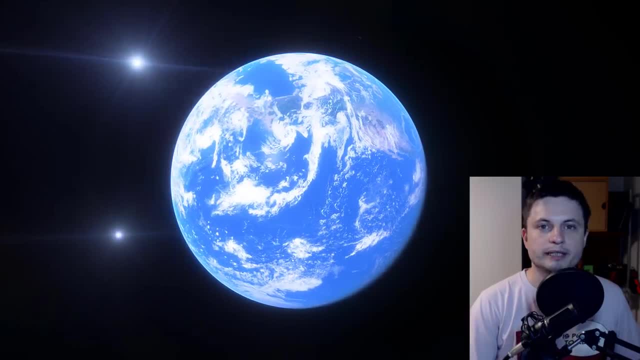 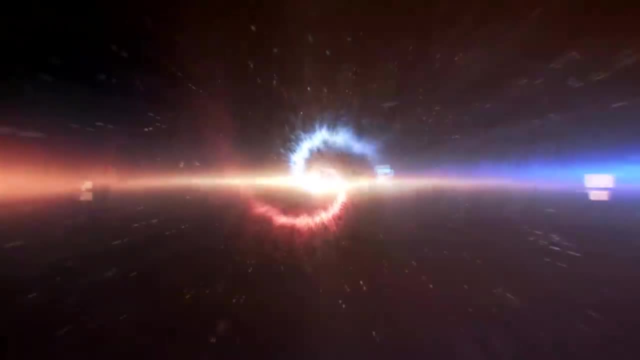 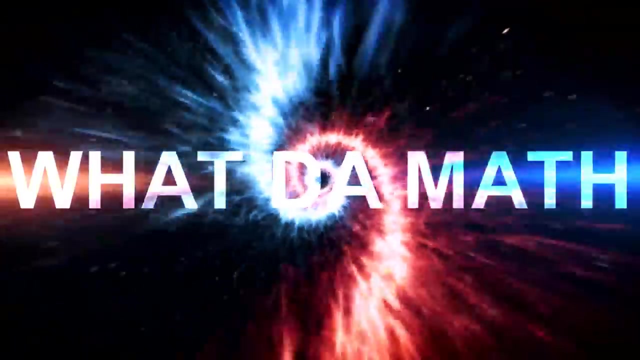 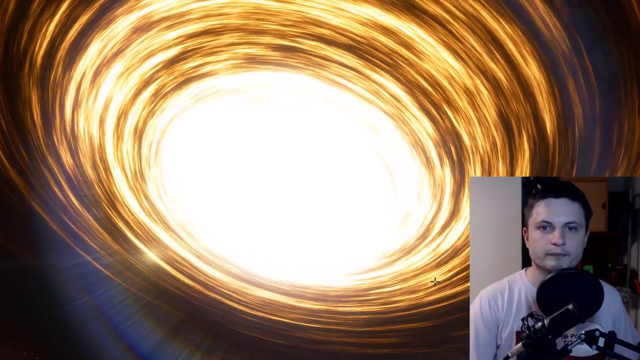 Hawking radiation, how black holes evaporate and disappear. So let's talk about this and welcome to What The Man. Now, you may already be familiar with the idea of black holes and how they work and what's around them and so on, and if not, you may want to check out some of the videos on the channel, where I do. 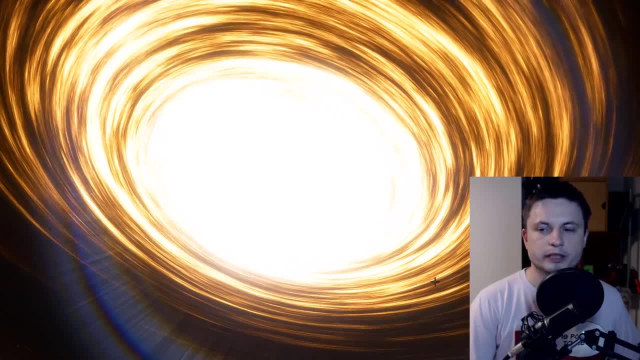 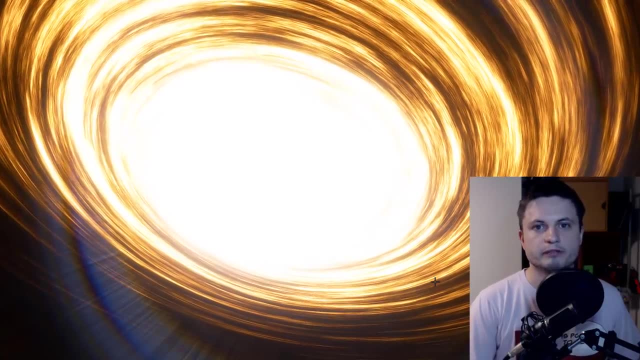 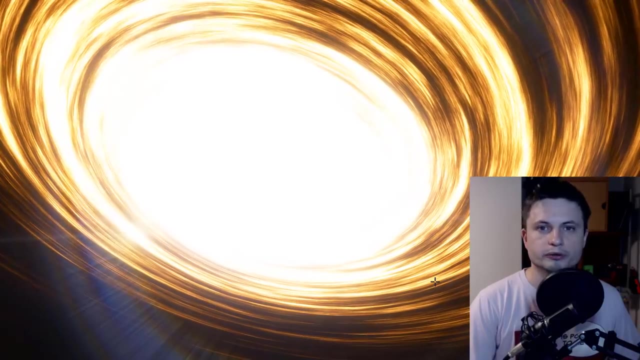 explain this in a little bit more detail, but in this particular video we're actually talking about their disappearance. So current understanding of black holes, based on the late Stephen Hawking and his book that was written about 40 years ago, is that eventually all black holes in our 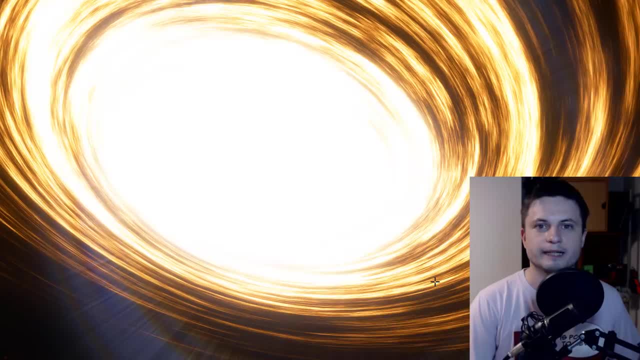 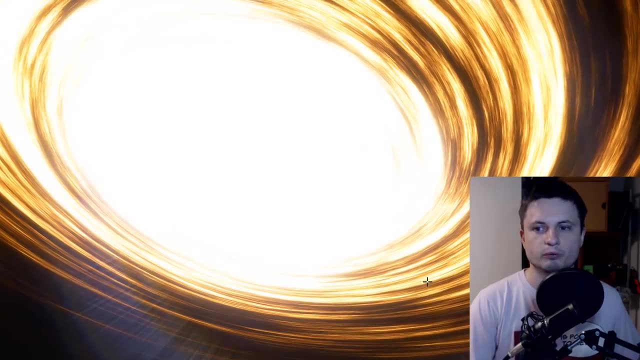 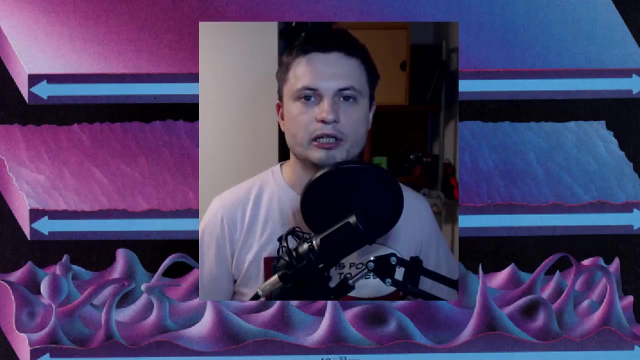 universe will actually disappear and eventually there will be nothing left except for just some energy and some leftover radiation. Now, how exactly does this work and what exactly happens around these monsters? Now we actually need to start our understanding of this phenomenon with the idea of energy in vacuum or, essentially, where there's like literally nothing. So this is. 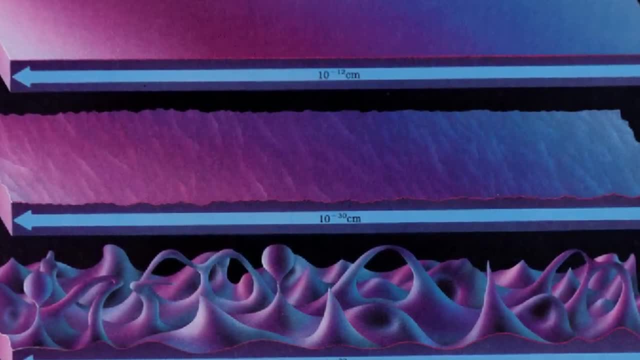 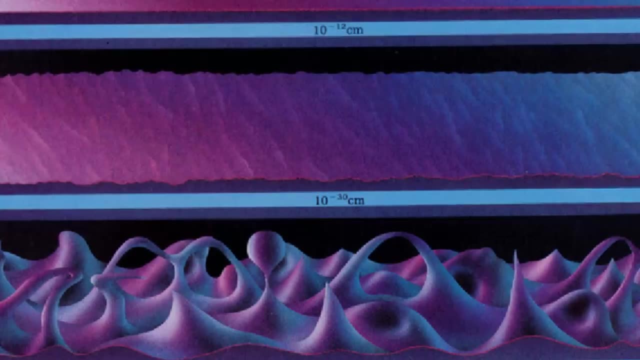 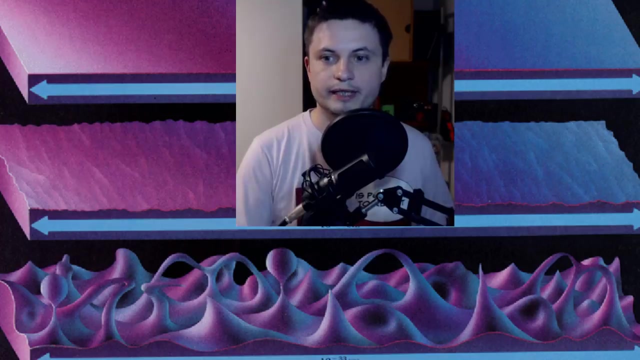 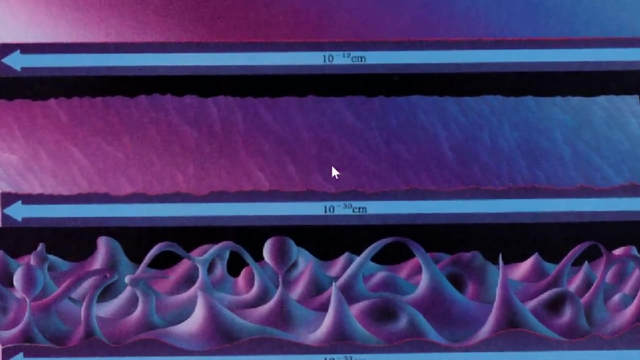 essentially completely empty space, and the modern understanding of this empty space is that there is no way for us to have zero energy in anywhere. You cannot possibly have completely accurate and completely measurable energy in any kind of space, no matter how empty it is. So as you kind of zoom into empty space you'll realize that there is a lot of stuff. 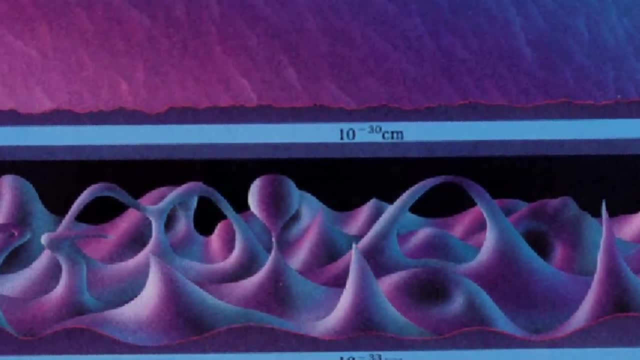 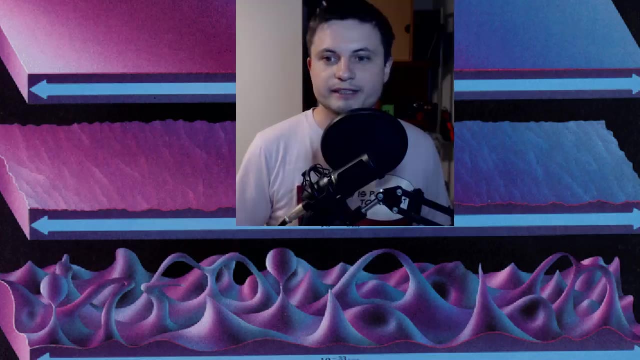 going on there. that was not actually visible, But here's the thing: as soon as you start observing it, there's this inherent time energy uncertainty that makes it impossible for us to know what exactly is happening there And to measure it to a very precise level, And this is essentially what's known as the 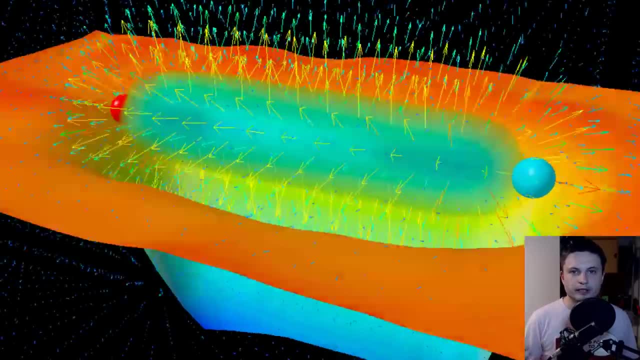 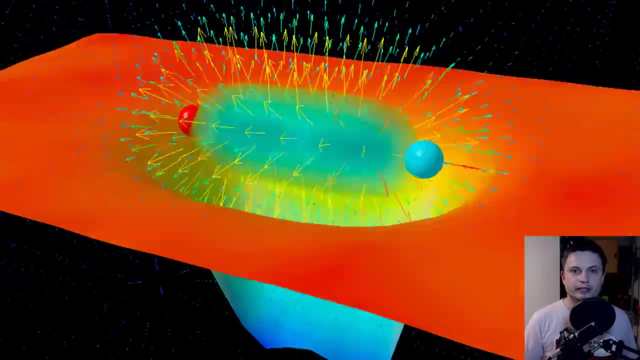 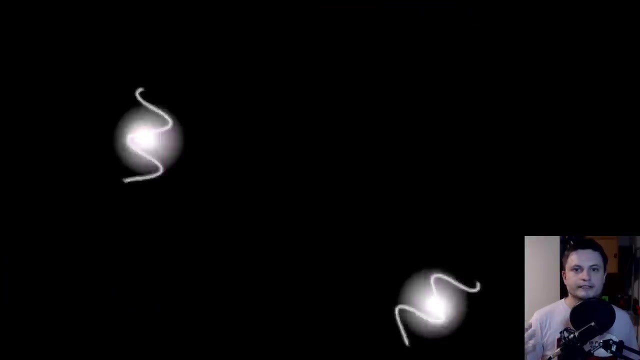 uncertainty principle. Even in completely empty space, there's actually always something going on and, specifically here, what you see on the screen is essentially that activity. There is always particles that are being created and destroyed, created and destroyed, created and destroyed- A slightly easier way of visualizing this is right here. So at any time in space and any space, even, 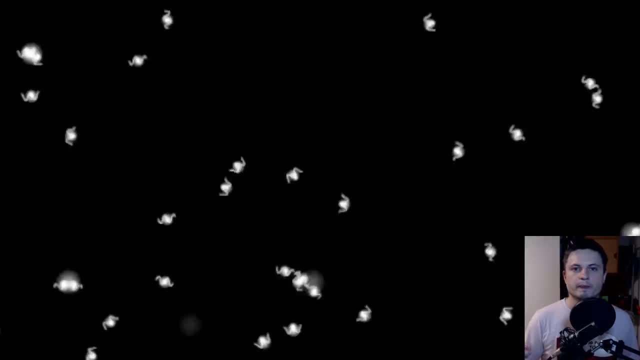 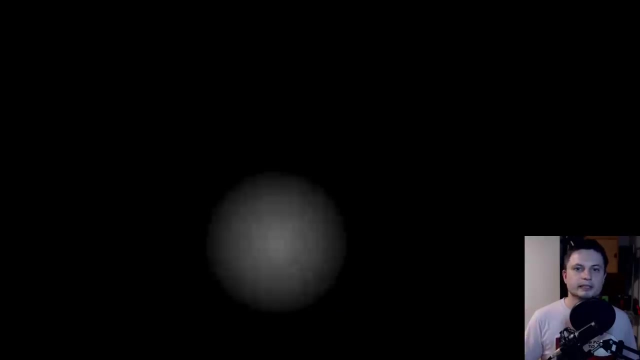 you have these virtual particles and antiparticles popping in and out of existence and creating this kind of a noise. that's always there, And our understanding of these particles and antiparticles is that they only do this for a very brief period of time and they completely disappear. 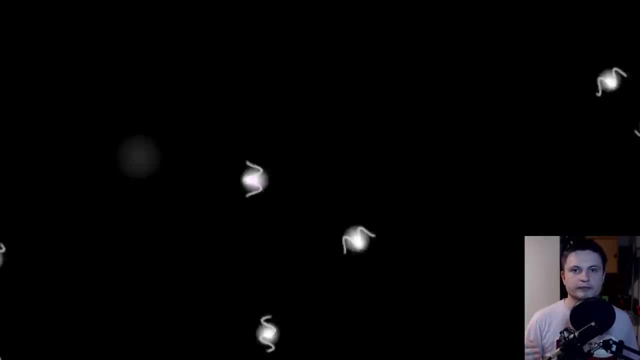 essentially keeping the overall state of space at an average zero. Now, at the same time, this becomes even more unusual and even more pronounced. that's what the ultimate identity of space is, So essentially more pronounced in a space around any kind of a supermassive object. So in other words, 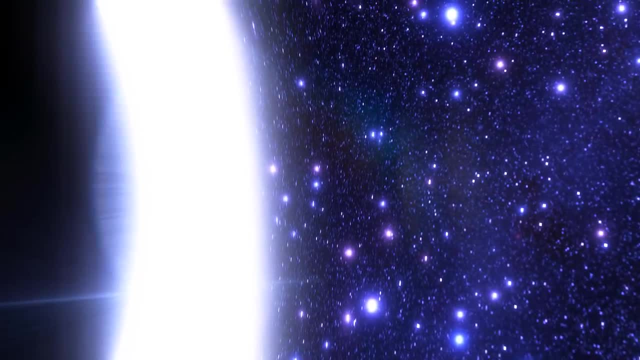 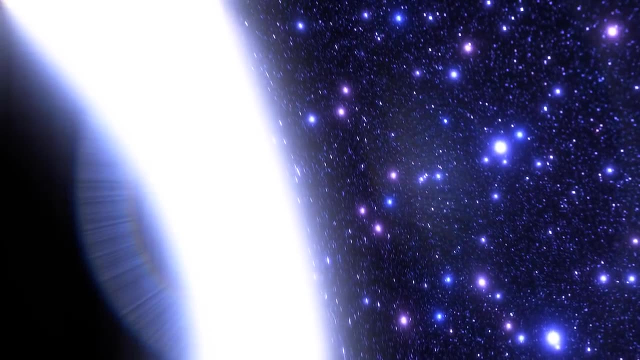 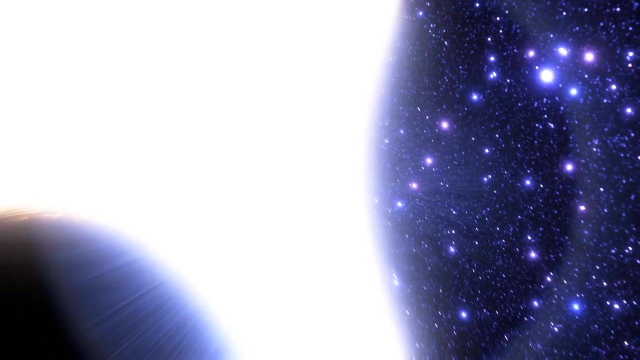 when the space is curved, like you see right here, right at the edge of the event horizon of the black hole, the actual particle interaction and the creation of these virtual particles and antiparticles increases dramatically. And so in curved space, the activity that you see on the 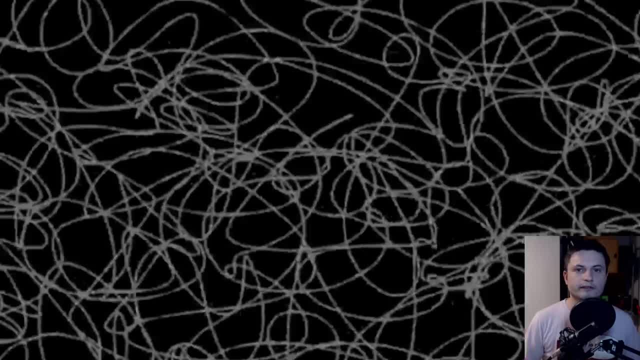 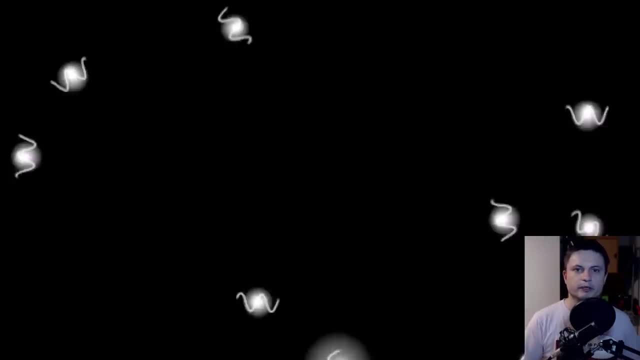 screen right now increases by essentially a very, very, very large margin, So it becomes a lot more prominent. The more curved the space is, the more likely these particles and antiparticles will start popping in and popping out of existence, And there's actually a very, very sort of difficult. 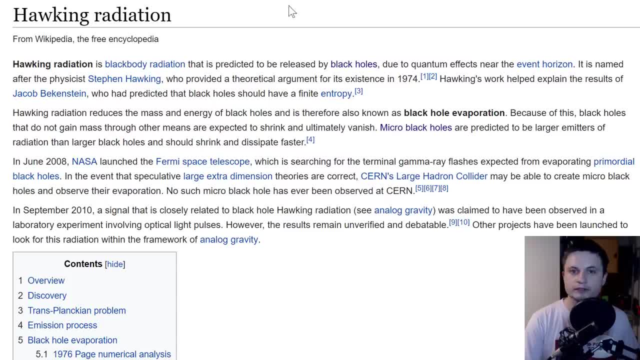 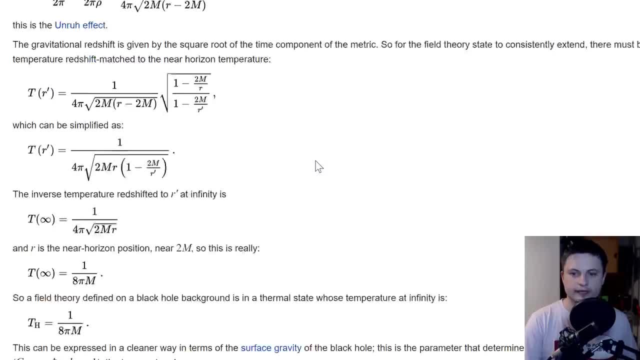 mathematics that explains this And the explanation itself is actually publicly available right here on the Wikipedia of Hawking Radiation. The actual mathematics is explained right here And all of the formulas are given to you. So if you are comfortable reading the math, you can actually read through this to see if you can. 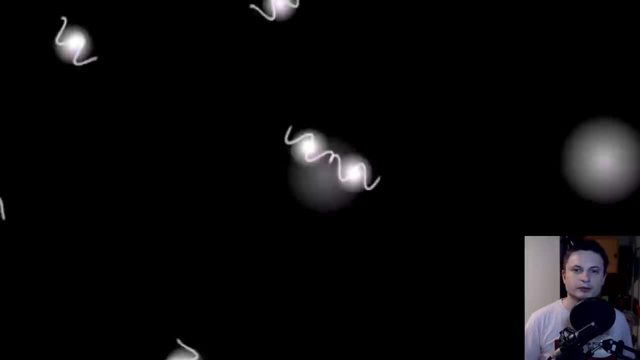 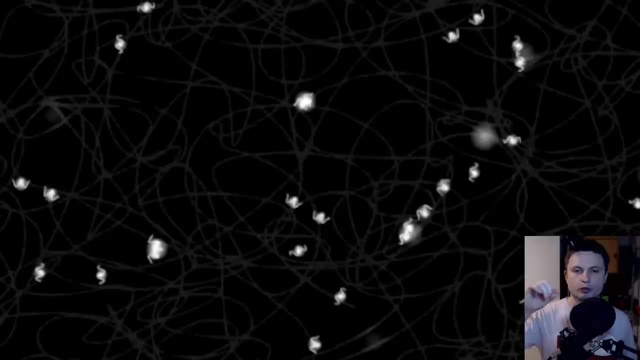 understand what's going on, But for those of us who are not really into reading math, that's the idea right here in this picture. Now, what about the black hole? So what if you actually have a black hole that has this curved space around it? And how does it all relate to black hole? 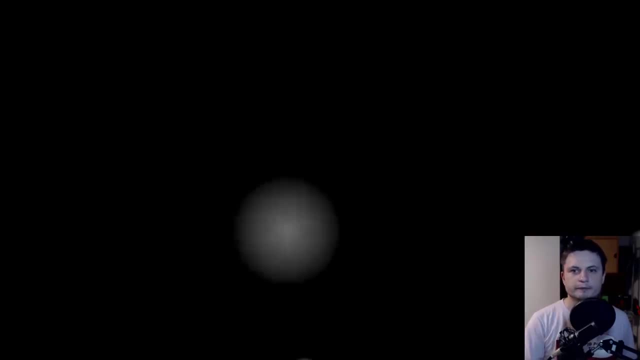 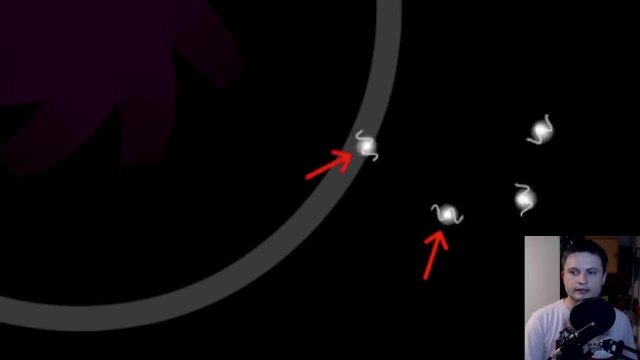 evaporation. Well, as you can imagine, if you actually find the location around the black hole, where the space is curved and also where, essentially, the event horizon starts- which is right here- at some point in time the particles or these virtual particles will create in such a way where one of them, either the particle or the 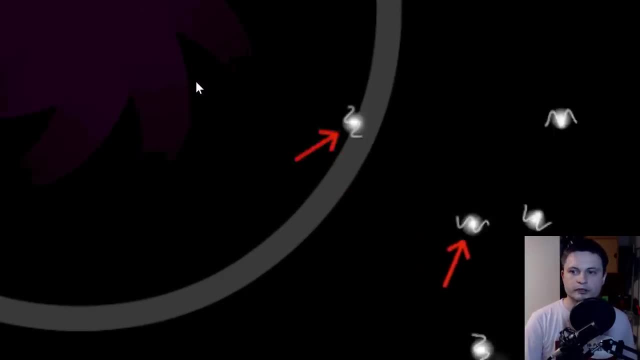 antiparticle will actually fall into the black hole because it just can't escape the gravitational pull. The other particle will have a chance to escape and will actually start sort of flying away from the black hole And, if by any chance, at the same time. 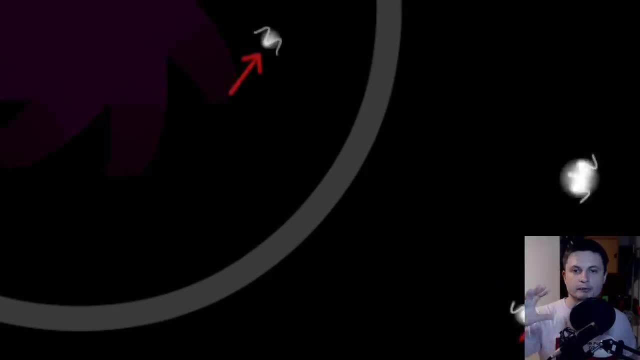 another pair of particles and antiparticles does the opposite. So let's just say this is the particle escaping and another antiparticle starts escaping at the same time, And then these two objects collide outside of the black hole. they will then, from being virtual particles, will. 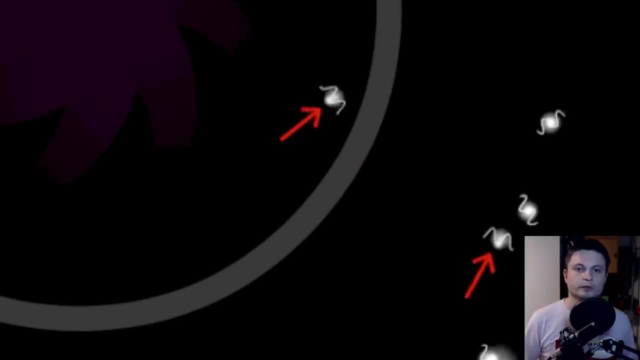 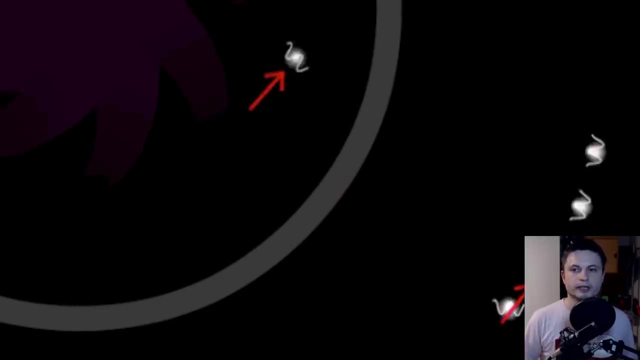 actually turn into real two photons of energy. So in other words, these virtual particle antiparticles will turn into real photons. They will emit some energy, But the way that our universe works is that you can't just create energy out of nothing. As a matter of fact, energy and mass are related, And so, because there's a 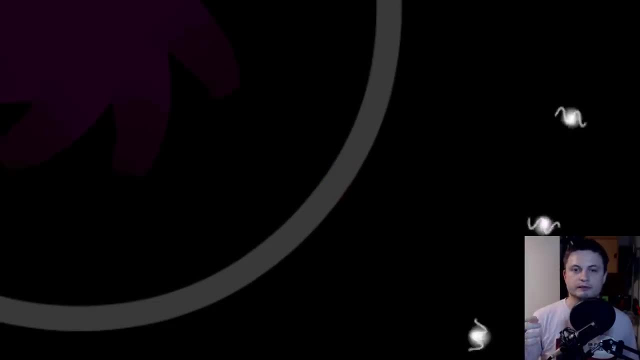 conservation of energy. here we need to actually be cycling this energy out of somewhere. And well, guess where it's coming from? It's coming from the black hole itself, And so these photons that will be escaping from this black hole will actually have a certain temperature. they'll have certain 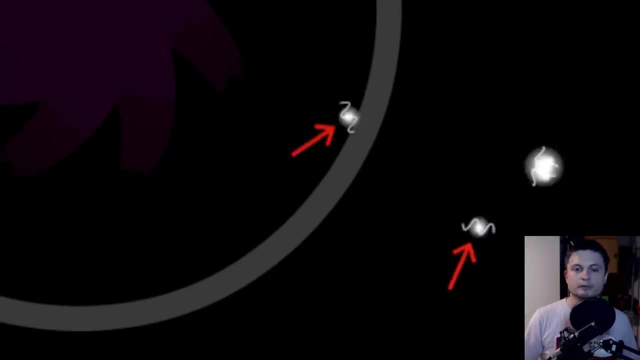 energy, and they'll be emitting this energy out of the black hole pretty much continuously, thus creating a kind of a black body radiation that you would expect from a typical object like, for example, a planet or even a star. And this formula to calculate the temperature of a typical black hole is also right here on. 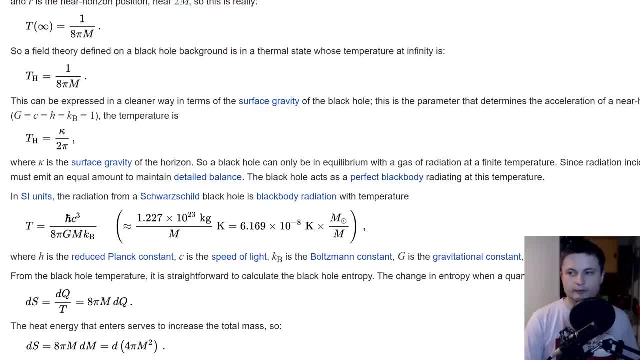 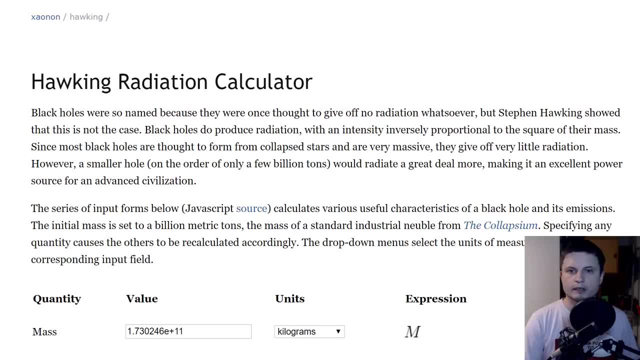 Wikipedia. This is actually how you can calculate it. Now, if you're not really a person that likes to dig into math and calculating things, here's a website that does it for you: The Hawking Radiation Calculator, created by Jim Wisniewski, whose website is in the description below. 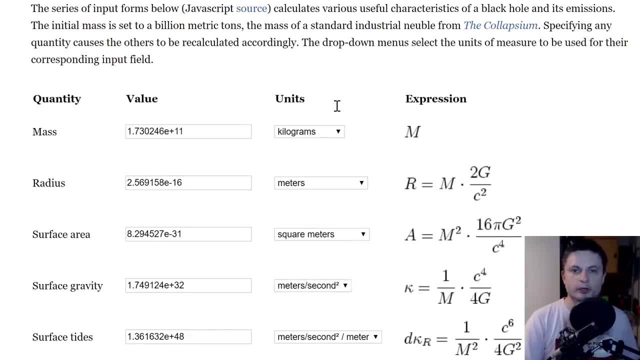 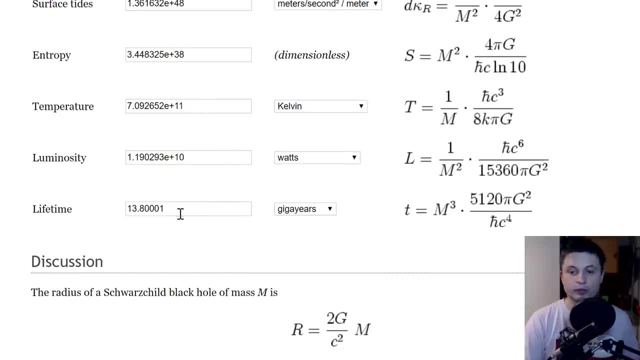 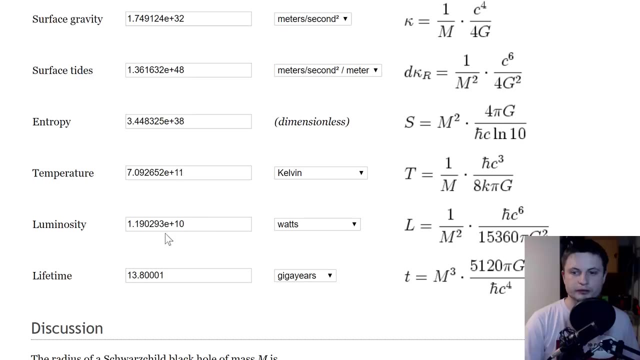 essentially allows you to calculate pretty much every single parameter of a black hole by just inputting the mass or the radius or the surface area or the actual lifetime that you would like to find out, and then kind of calculating things like, for example, temperature, luminosity. 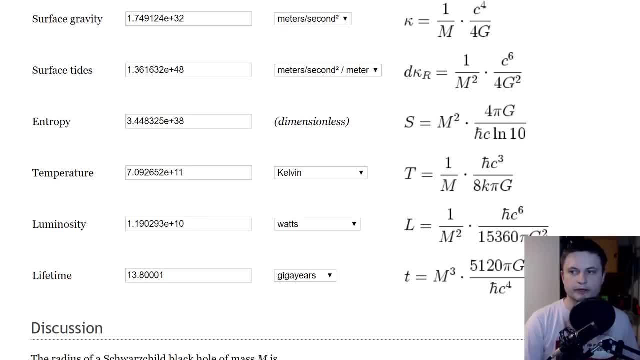 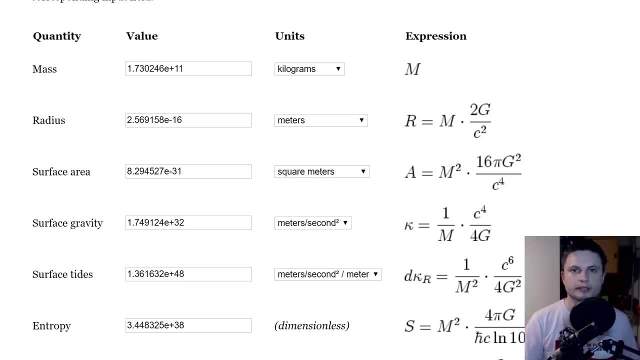 and so on. So this is a beautiful website that I've previously mentioned in one of the videos as well, and does all of the math for you. So like, let's just say, for example, for our own supermassive black hole, Sagittarius A star, if we input the actual mass of the black. 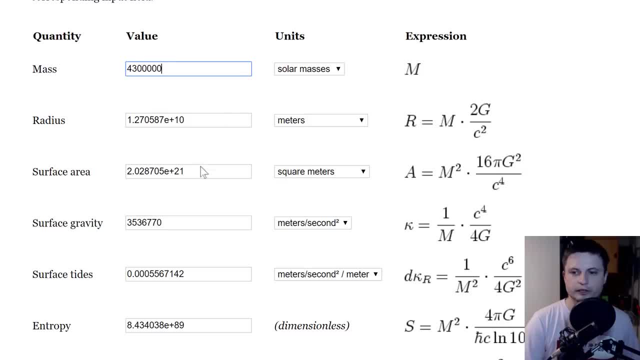 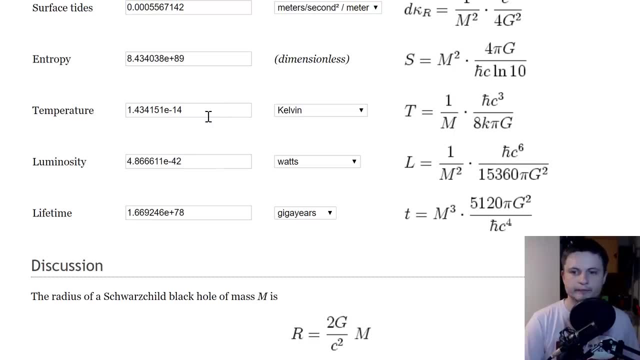 hole and press enter. it will calculate the radius for us, it will calculate the area, the gravity and, most importantly, it will also calculate the temperature that the supermassive black hole is emitting right now, the luminosity that it has and its total lifetime. So this is how. 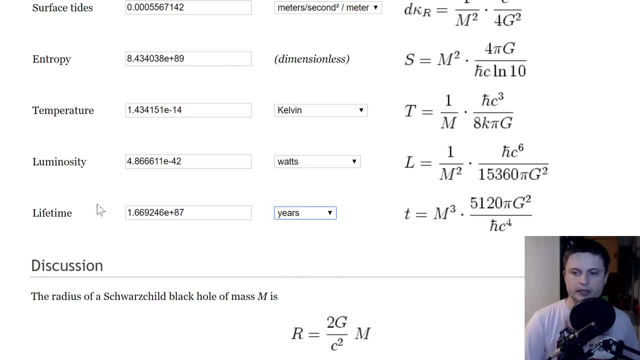 many. okay, this is giga years. this is how many years our black hole will actually live for. So it's 1.7 times 10.. to the power of 87. So that's 87 zeros. It's a lot, a lot of years And, as you can imagine, 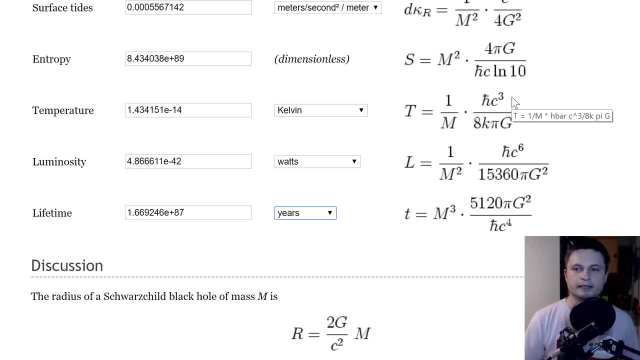 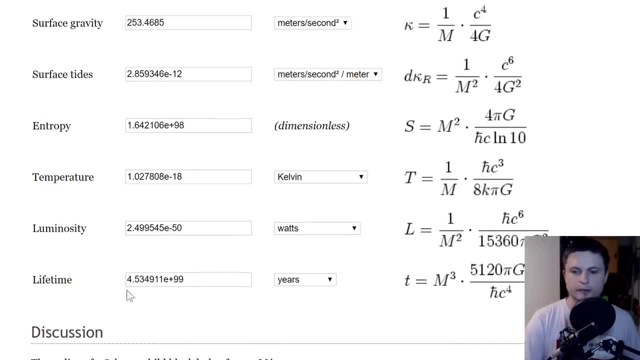 the more massive the black hole, the more it will live, and thus some of the more massive black holes we've discovered so far may actually live up to about 4.5 times 10, to the power of 100 years. So basically, that's 100 zeros. Now this number is so big that it's currently 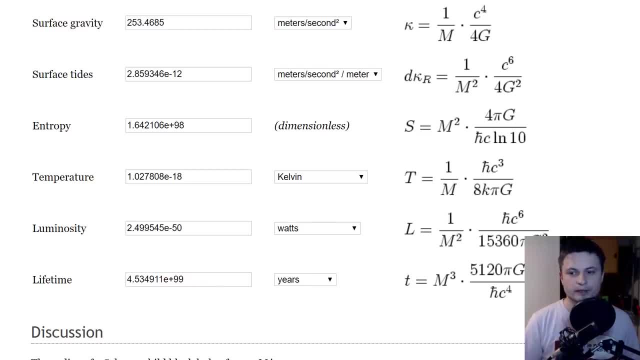 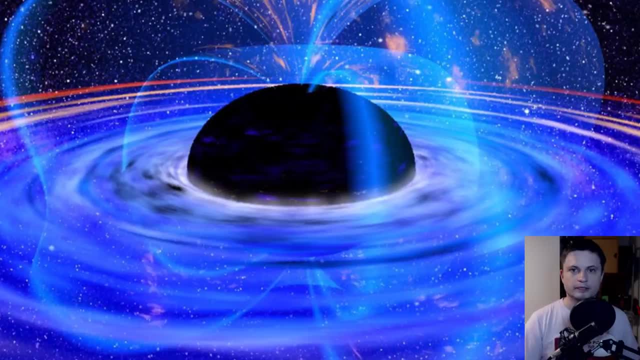 estimated to be even longer than the potential age of the universe. but if the universe lives a little bit longer, then this is the time it takes for the last black hole to evaporate. And so, as these particle-antiparticle pairs kind of steal the 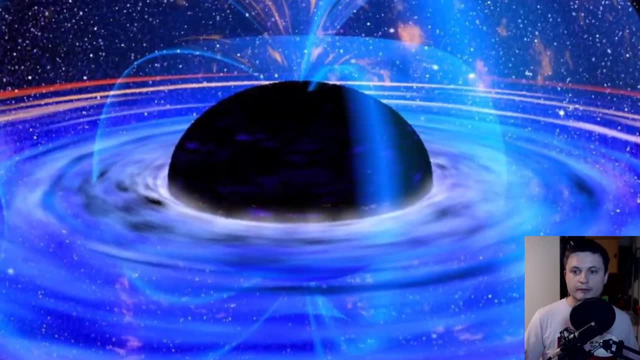 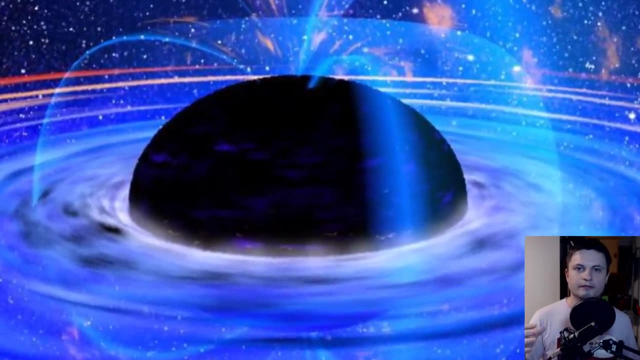 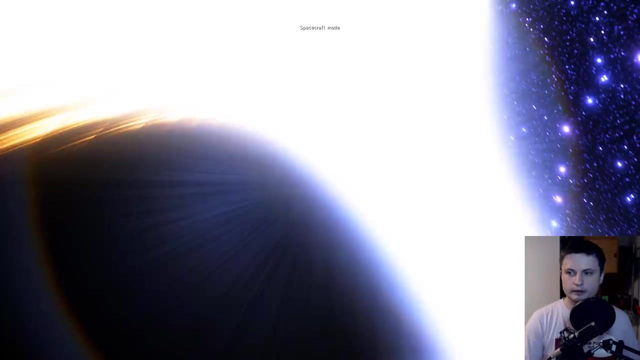 energy and the mass of a black hole. over time, they'll actually start doing this more and more often, And that's because a smaller black hole will actually have much higher curvature around its event horizon. The more massive and the bigger the black hole, the less 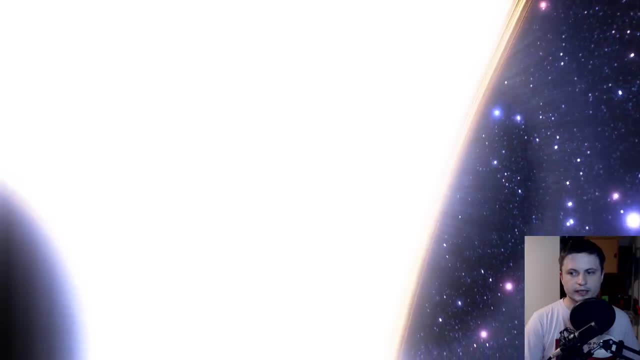 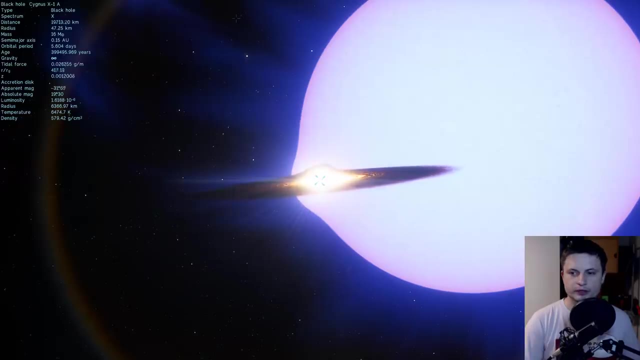 space curvature it gets. So this supermassive black hole right here doesn't actually curve space as much, But a much smaller black hole, like, for example, Cygnus X-1 that you see right here, which is actually one of the most well-known solar mass black holes, has such a high curvature. 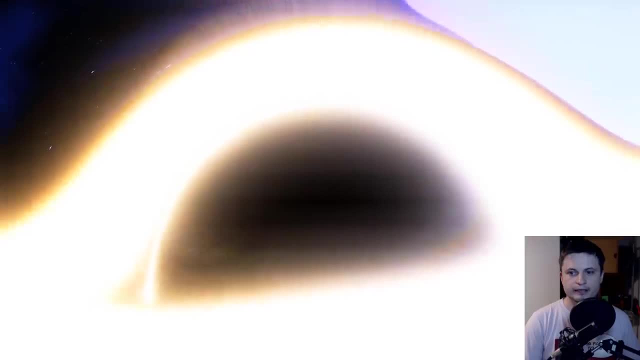 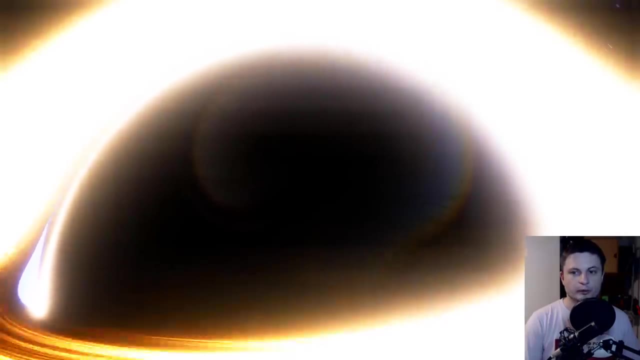 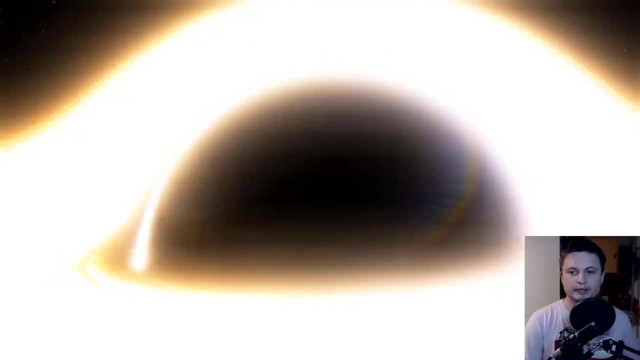 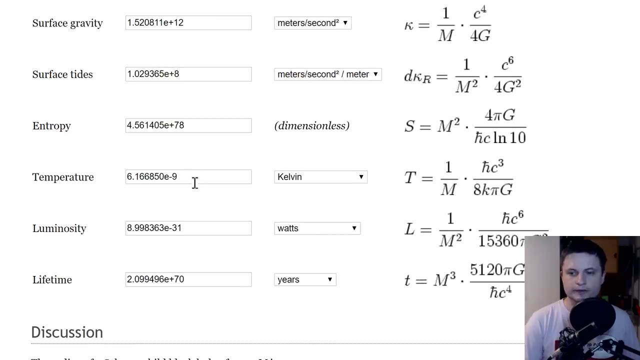 are still actually kind of minuscule. So if we were to input its mass here, which is maybe roughly about 10 solar masses, you would find out that, first of all, its temperature is still very low. It's not even one degree, It's like 0.806,. 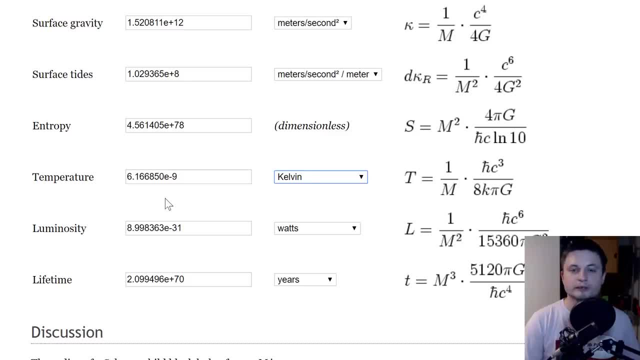 which is a tremendously low number. It's still really, really, really, really, really cold, and its luminosity is very low and its lifetime is still pretty long. However, if you were to start hypothesizing about much smaller black holes, like, for example, something similar to the: 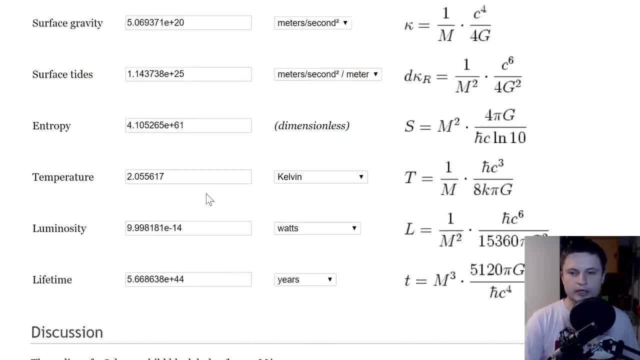 mass of the Moon, or basically about one hundredth of mass of Earth. at this point it now has temperature of 2 degrees 2 degrees Kelvin, that is, which is still approximately minus 271 Celsius or minus 455 Fahrenheit, but the lifetime becomes much shorter and the luminosity also increases. 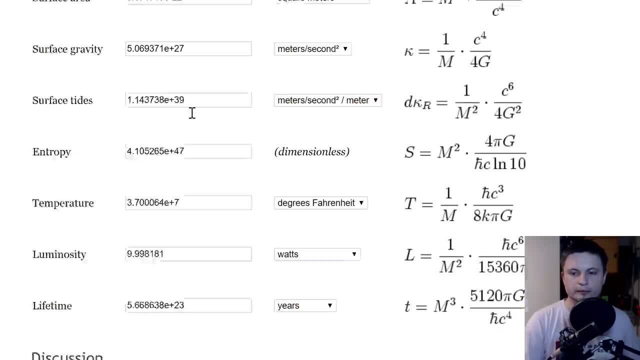 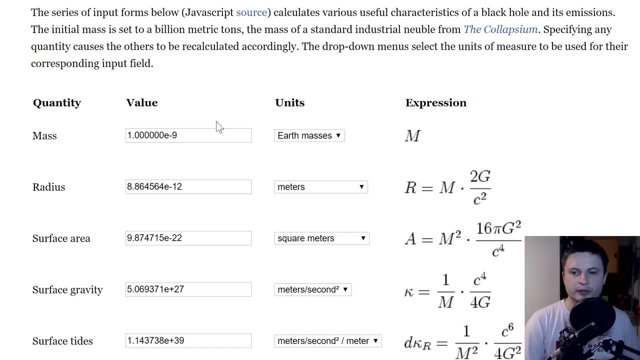 a little bit, And at some point we can actually reach a number of degrees- and that's why we're number- where the black hole itself will start emitting quite a lot of temperature, but at some point you can actually find a number here that will essentially create what's known as a mini. 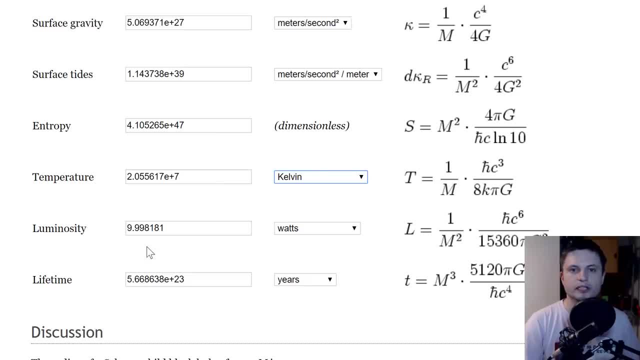 black hole where the luminosity becomes quite obvious. You can actually start seeing the black hole shine. essentially, so it's no longer really a black hole. It's literally the opposite of a black hole, and its temperature becomes really high and its lifetime becomes a lot lower. as 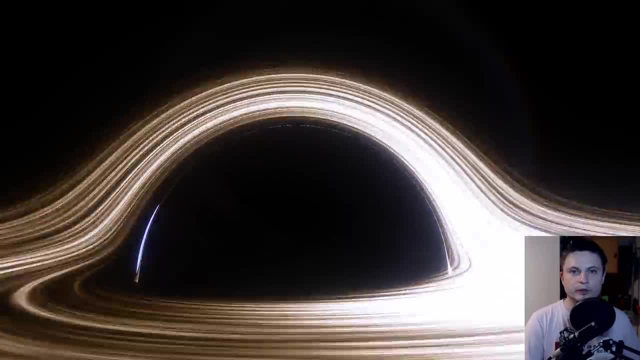 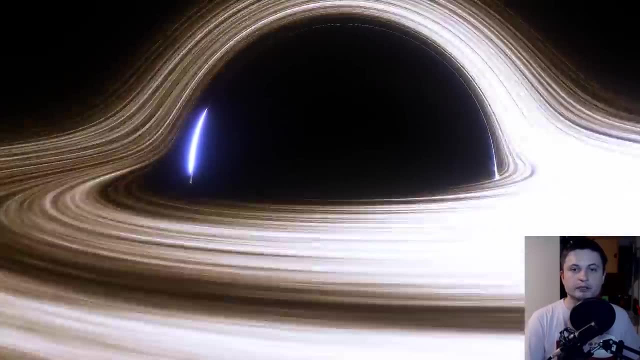 well, Now we'll actually talk about the black hole in a little bit, but before we do that, I want to talk about mini black holes in another video, where I'm going to also talk about how you could produce energy using these objects. but the idea of a black hole evaporation has a potential. 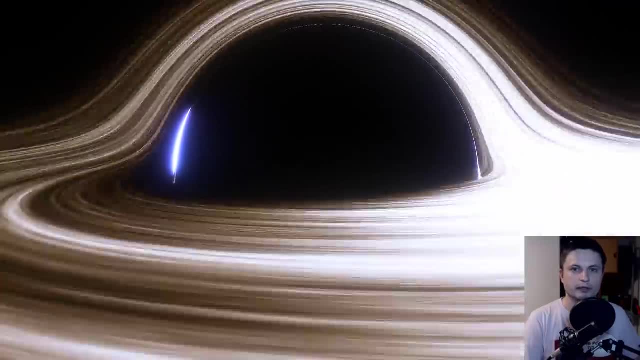 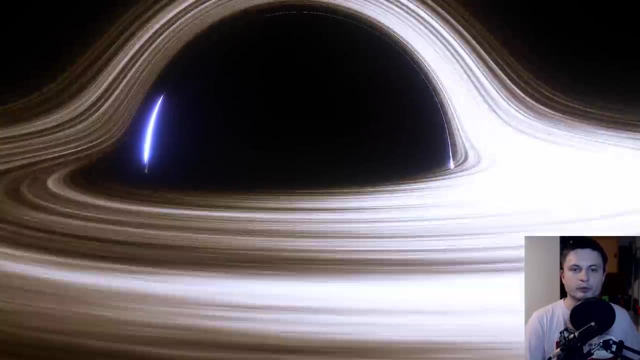 of creating quite a ridiculous amount of energy for the humankind. As a matter of fact, this is maybe, or hopefully will be, one of the biggest discoveries of the 21st century. I hope we can actually find a way to harness this energy, and I really, really hope that we are at some point. 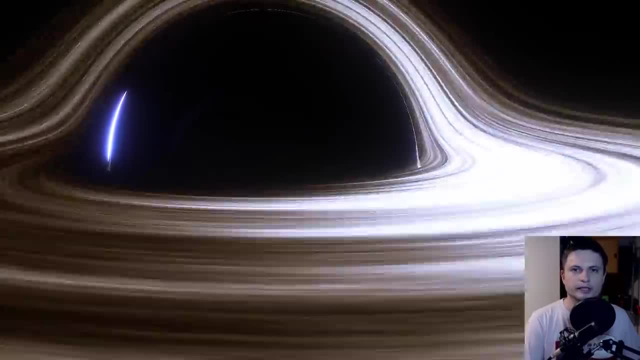 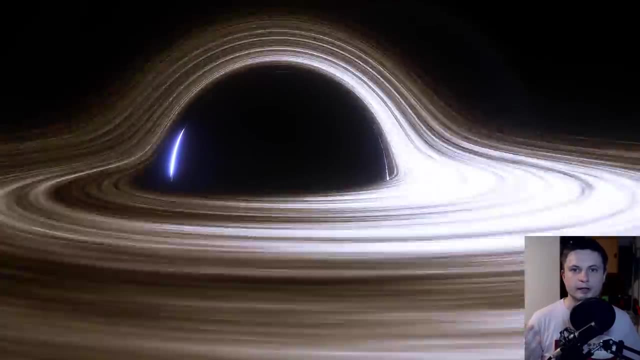 able to manipulate these extremely exotic objects And other than that. that's really all I wanted to mention in this video. I wanted to explain the idea of Hawking radiation and how black holes evaporate, and I also wanted to show you this website that allows you to calculate pretty much everything by yourself. So in one of the next 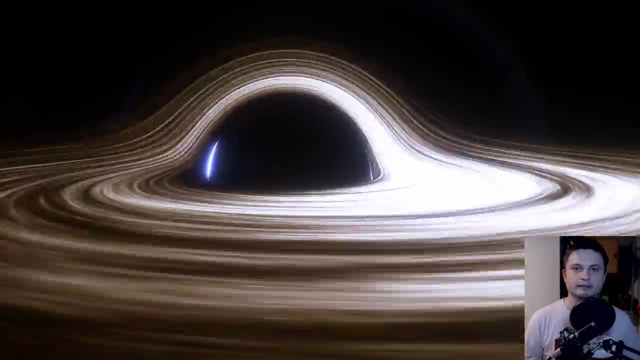 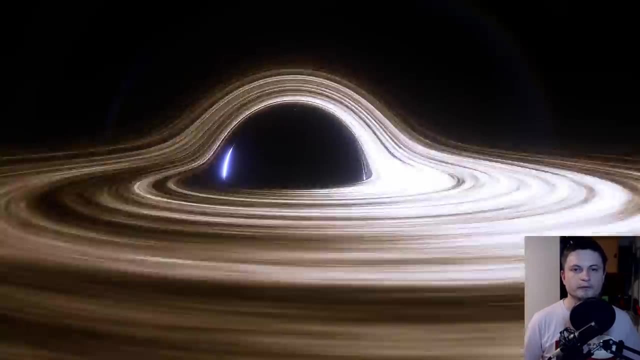 videos, we'll explore the idea of mini black holes and the unlimited energy that they can create for us. So do come back and watch the video tomorrow and you might learn something you didn't know, And also subscribe, if you still haven't. share this video with someone who wants to learn about.